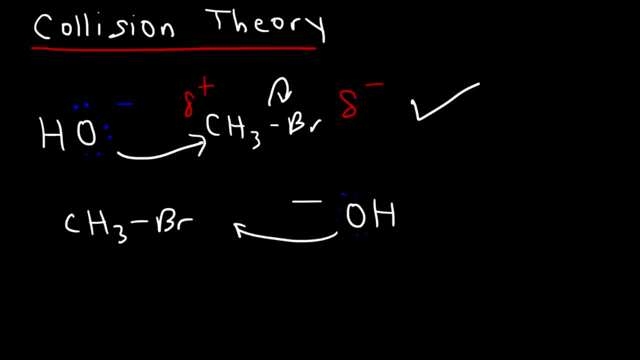 Well, the reaction's not going to happen. Hydroxide is repelled by the partial negative charge of the bromine atom, And so when two negative charges come together, they're going to feel a force that's going to repel them. 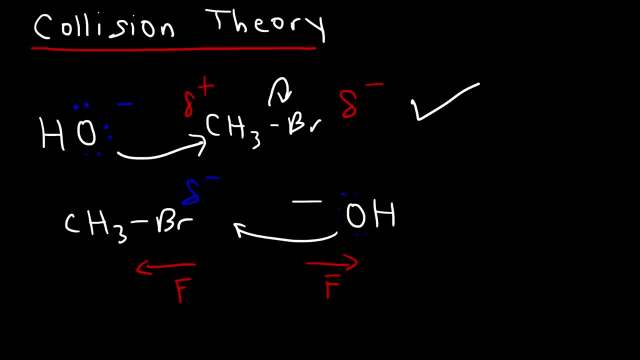 And so that's going to prevent the reaction from occurring, Whereas when hydroxide attacks from the carbon side, the negative charge on the hydroxide is attracted to the partially positive charge on the carbon atom, And that electrostatic force of attraction accelerates them together, which favors the collision of those two molecules. 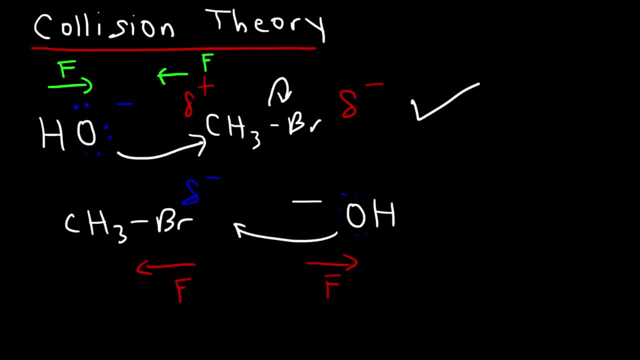 And so if the two molecules do not have the correct molecular orientation, the reaction's not going to happen. But if they collide with the appropriate orientation, then the reaction's going to happen. So in order for a reaction to occur, molecules they have to collide. 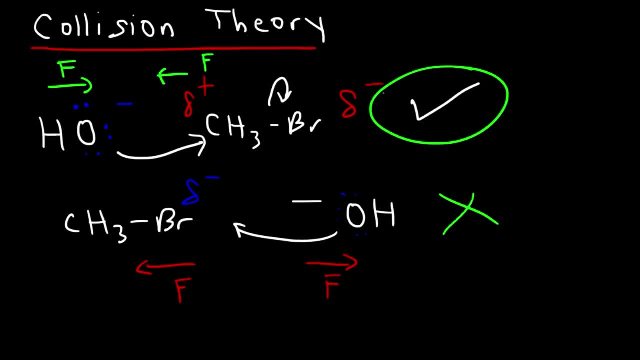 And two, they have to collide with the right orientation. Now, the third thing is that they need enough energy, Because if the temperature is low, even though these two may be attracted to each other, if the hydroxide ion doesn't move with enough momentum, 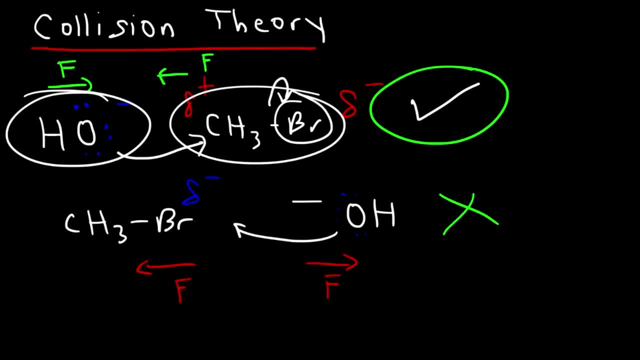 it's not going to be enough to knock off this bromide ion, So it has to have enough energy to attack the carbon atom and expel the bromide ion out of that reaction to create methanol. So there's three things that is required for a reaction to take place. 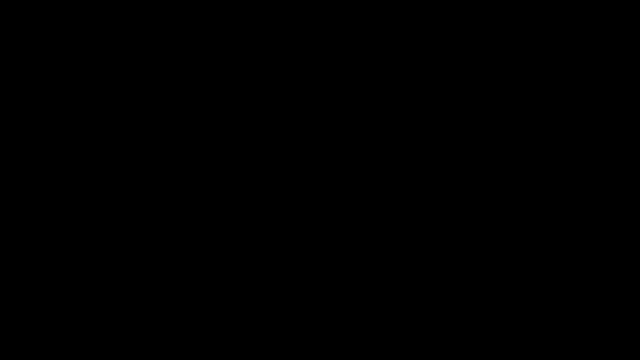 The molecules must collide and they have to collide with the right orientation and they have to have sufficient energy to break some bonds and form some new bonds. Now this leads us into energy diagrams. So on the y-axis is the energy of the system, on the x-axis is going to be the reaction coordinate. 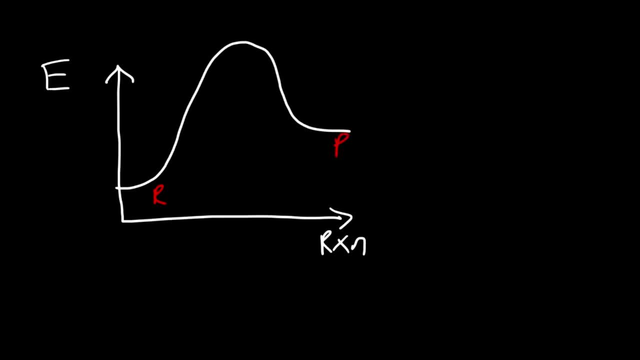 Here we have the reactants and here we have the products. The top is the transition state, also known as the activated complex. In order for this reaction to occur, the system has to have enough energy to create a reaction to the reaction. 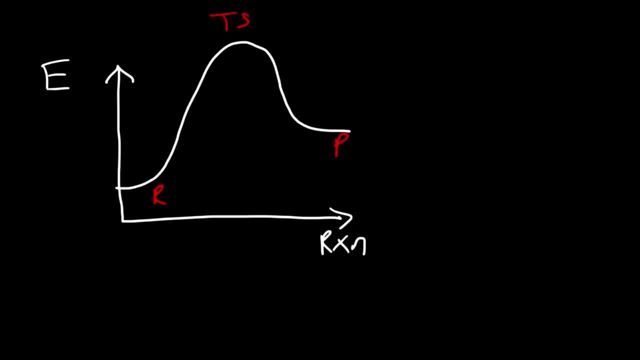 The system has to have enough energy to create a reaction to the reaction. The system has to have enough energy to create a reaction to the reaction. The reactants need to gain enough energy. The reactants need to gain enough energy to create a reaction to the reaction. 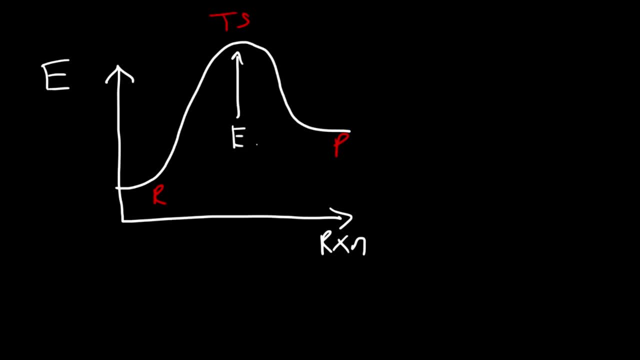 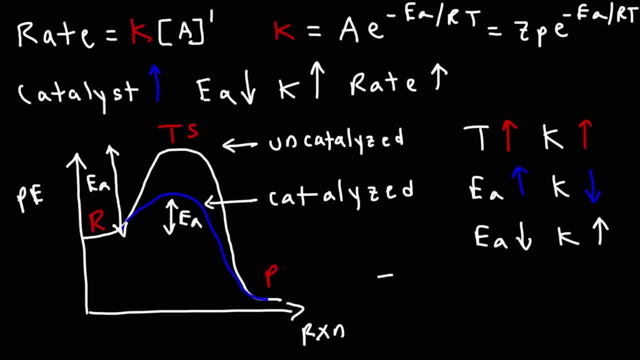 If the reactants do not have enough energy to overcome the activation energy, the reaction will not happen. If the reactants do not have enough energy to overcome the activation energy, the reaction will not happen. So, to summarize, if we increase the concentration of the reactant, the rate is going to go up. 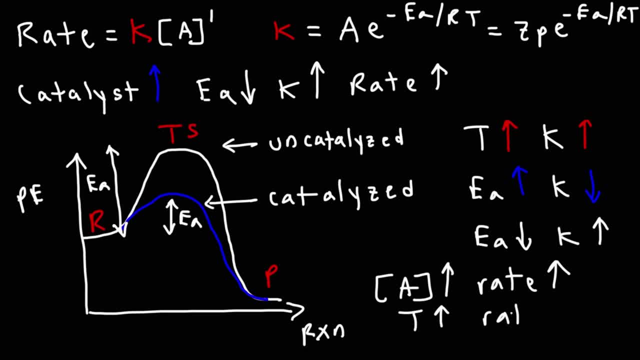 If we increase the temperature, the rate of the chemical reaction will go up, And if we add a catalyst, the activation energy will go down and the rate of the reaction will go up. So those are some different ways in which we can increase the rate of a chemical reaction. 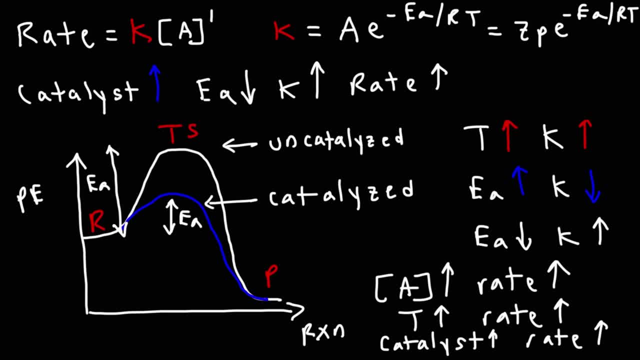 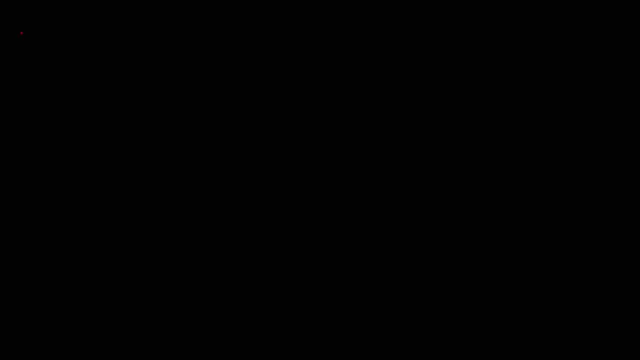 You can increase the concentration, raise the temperature or introduce a catalyst To speed up the reaction. Now let's write down some equations that you'll need to know in order to solve problems, So you're already familiar with this one. The rate constant K is equal to the frequency factor times E raised to the negative Ea over RT. 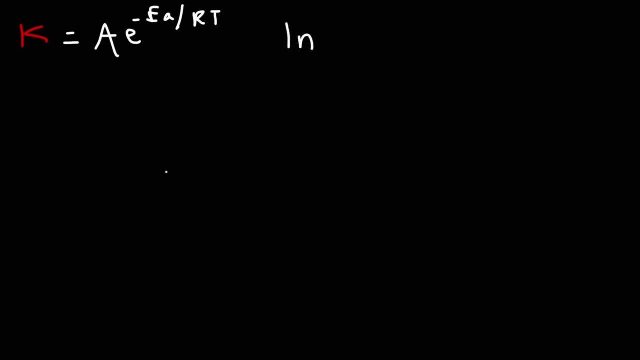 Here's another one that you should be familiar with: The natural log of the rate constant K. That's equal to negative Ea over R times 1 over T, plus the natural log of A. Now, in this form, this is written in slope intercept form. 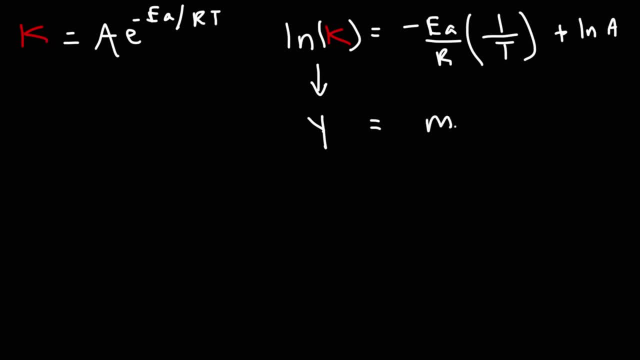 So Y corresponds to L and K, The slope M corresponds to negative Ea over R, X corresponds to 1 over T And the Y intercept B is L and A. So if you were to graph Y versus X, where Y is L and K, so we'll put that on the X axis, I mean the Y axis. 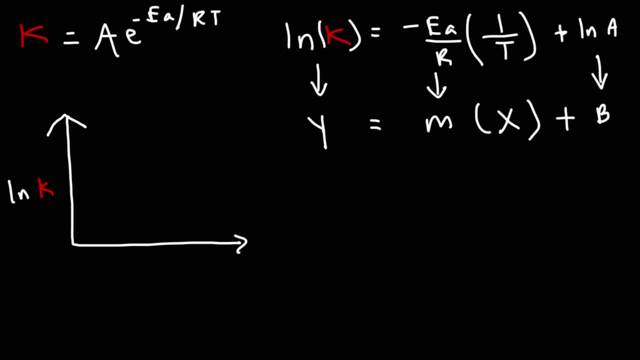 And 1 over T is X, so we'll put 1 over T on the X axis. You're going to get a graph that looks like this: It's going to be a straight line plot. But notice that this is a straight line plot. 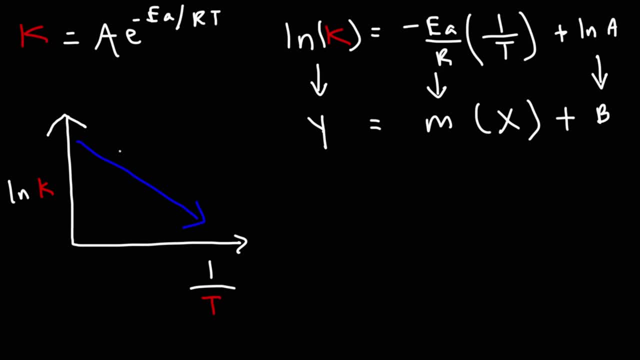 So you're going to get a graph that looks like this. So you're going to get a graph that looks like this. So you're going to get a graph that looks like this, But notice that the slope is negative. So the slope of this line is going to equal negative Ea over R. 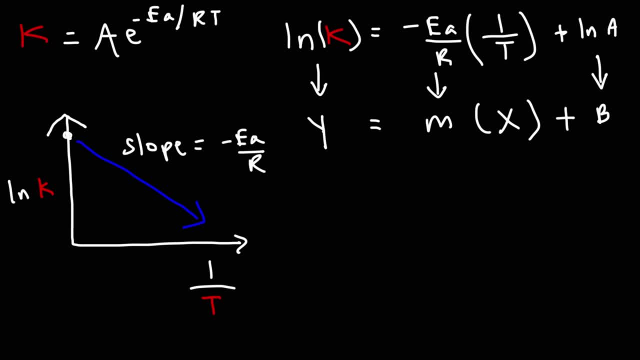 And the Y intercept, which this is where the graph starts from. that's going to be L and A. So for problems associated with this equation, if you have a plot of L and K versus 1 over T, just know that You can find the activation energy from the slope of the graph. 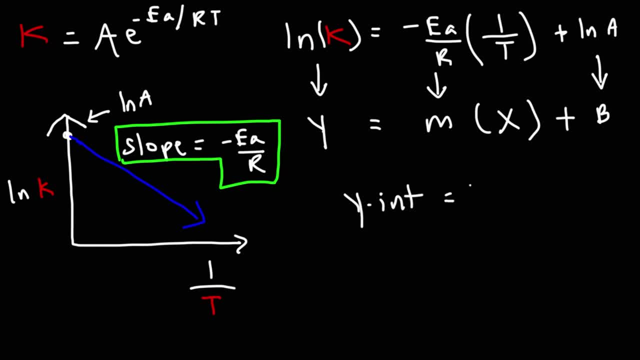 And the Y intercept is equal to the natural log of A, So you could find a frequency factor from the Y intercept. Now R is 8.3145 joules per mole per Kelvin. So because R has the unit joules and moles, the activation energy which is typically reported in Kelvin. 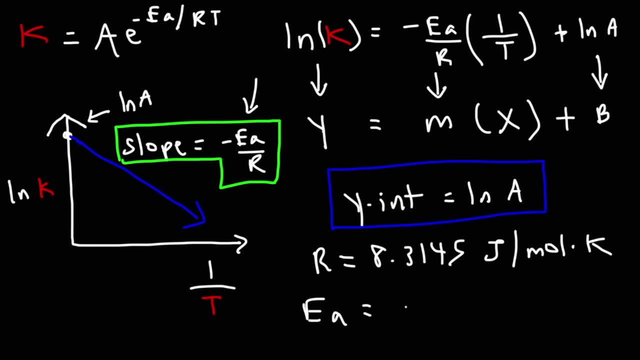 is going to be in kilojoules per mole. When you use it in these formulas, it needs to be in joules per mole, So you need to convert it. So when reporting the activation energy, you want your answer to be in kilojoules per mole. 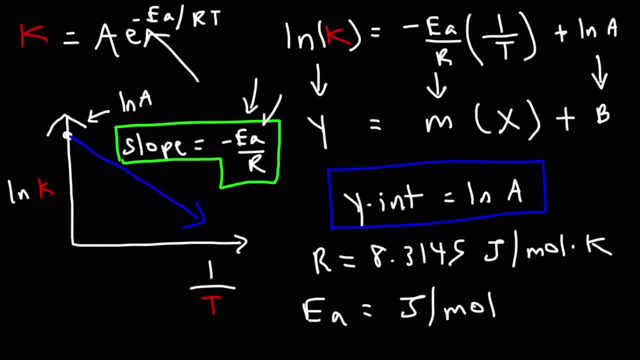 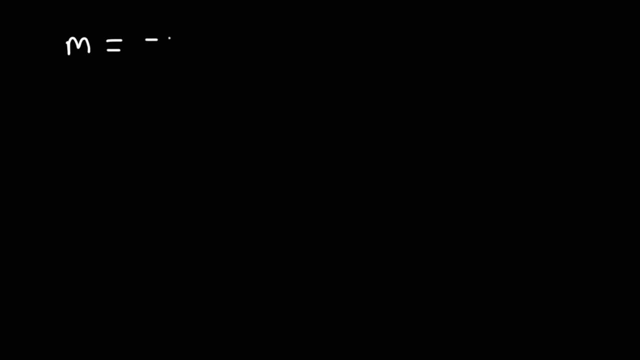 But whenever you plug it into one of these formulas, you need to convert it to joules per mole, So make sure to be aware of that. Now, the slope M is equal to negative Ea over R And the slope is Y intercept Y2 minus Y1 divided by X2 minus X1. 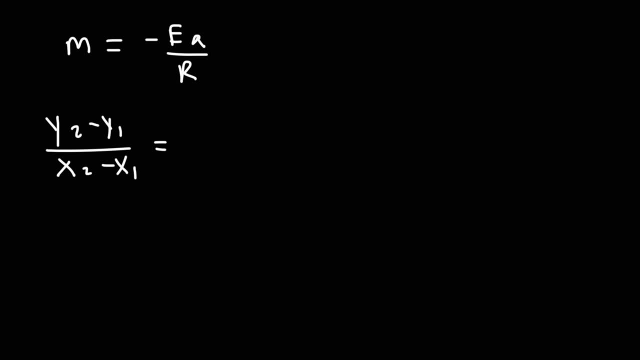 L and K is on the Y axis And 1 over T is on the X axis. So if Y is equal to L and K, we could say that this is L and K2 minus L and K1, all divided by 1 over T2 minus 1 over T1. 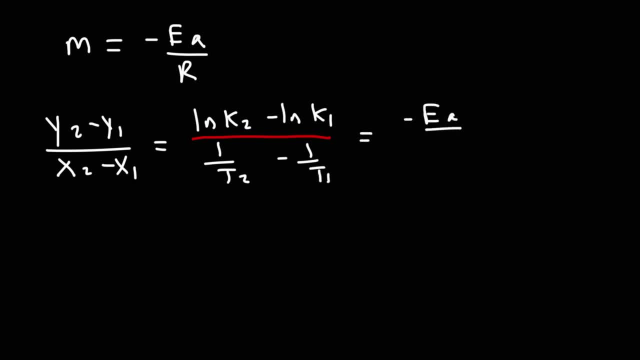 So that's going to equal negative Ea over R. Now let's say if we have L and K2.. L and A minus L and B. Using the property of natural logs or logs, we can convert this into a single log expression by writing it like this: L and A over B. 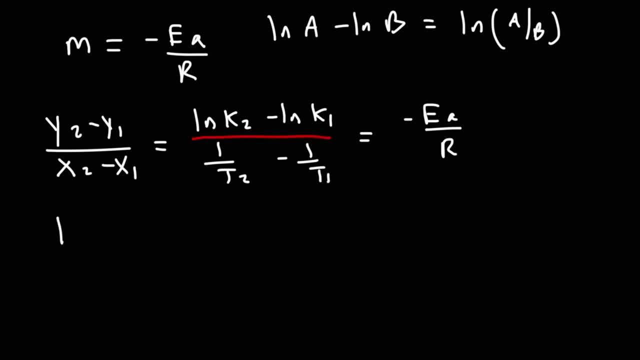 So we can write this as a single log expression as well. We can say that that's L and A. I mean, that's L and K2 over K1.. And this is 1 over T2 minus 1 over T1. 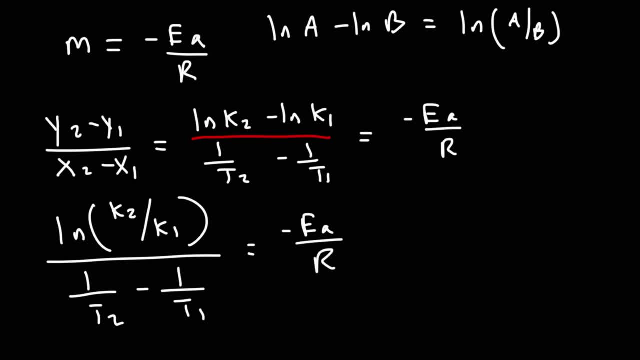 And that equals negative Ea over R. Now if we want to get activation energy by itself, we can multiply both sides by negative R. If we do that, R will cancel on the right side as well as the negative side And we'll get an equation for activation energy. 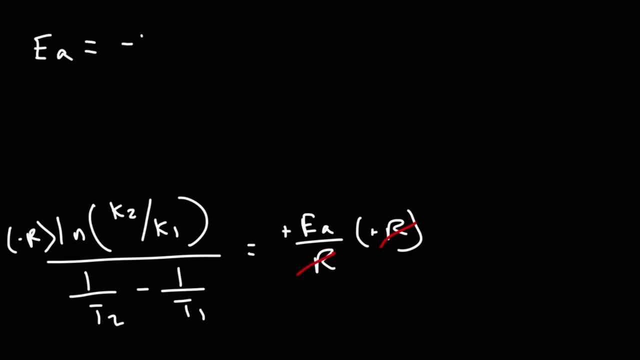 So the activation energy is going to be negative R. So the activation energy is going to be negative R. So the activation energy is going to be negative R. Ln. K2 over K1 divided by 1 over T2, minus 1 over T1.. 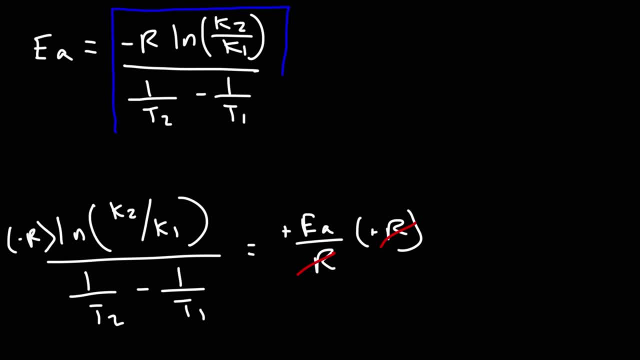 So you could use this equation to calculate activation energy. Now you might see a variant of this equation. Sometimes this negative sign will be distributed to 1 over T2 minus 1 over T1. And that will basically flip the order of T1 and T2.. 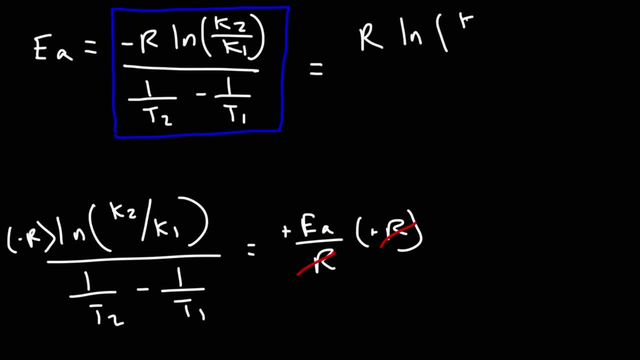 So this is also equal to positive R, Ln, K2 over K1. And if you distribute the negative sign, negative times, negative 1 over T becomes positive 1 over T1. And then here this will be negative, So minus 1 over T2.. 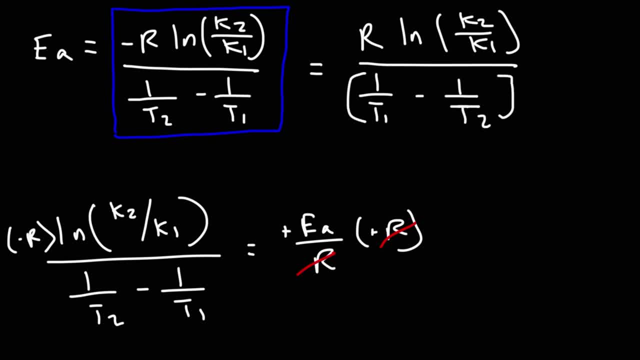 So you might see it in that format too. So just be aware of that. But if you have the negative sign, it's going to be 1 over T2 minus 1 over T1, instead of the reverse. Now let's go back to this equation. 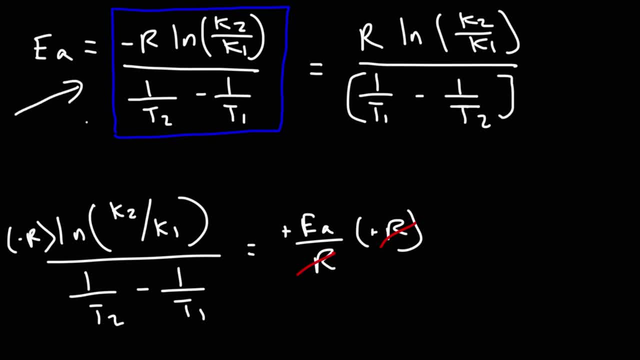 Make sure to write this equation, by the way, because you're going to need it to solve problems. Now, instead of multiplying both sides by negative R, Let's multiply both sides by This term. if we do that, we'll get a different equation. 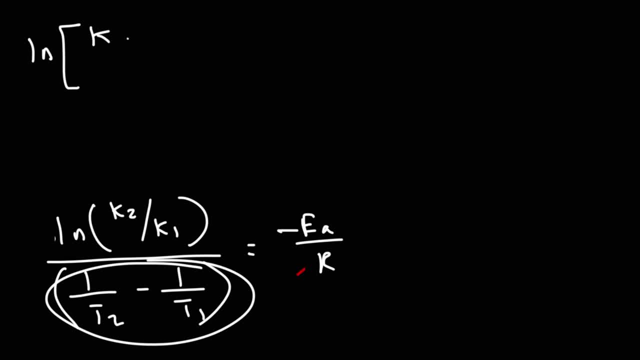 We'll get this one: Ln K2 divided by K1 is equal to negative Ea over R, And we're going to move this to the other side, times 1 over T2 minus 1 over T1. So that's another form of the Arrhenius equation that you might see it in. 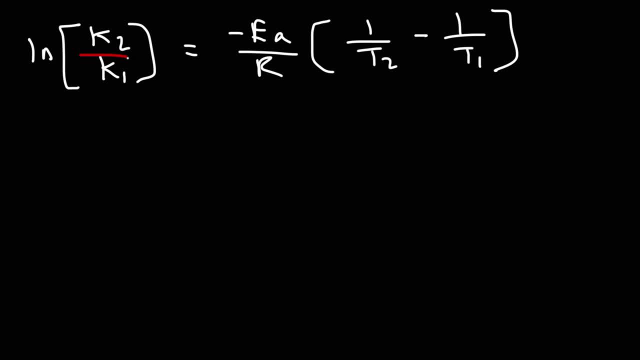 Now, what we're going to do at this point is we're going to put both sides of this equation on the exponent of E. So I'm going to put all of this on the exponent of E and all of this on the exponent of E. 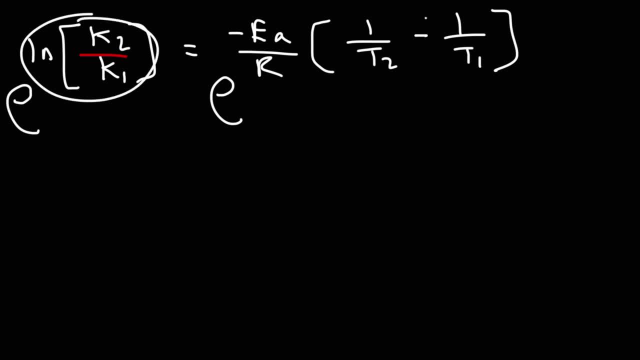 Because E is the same And these two are equal to each other. Both sides of this equation will be equivalent. Now, the base of a natural log is E, So on the left side, these two will cancel, And so we're just going to get K2 over. K1 is equal to everything that we see here. 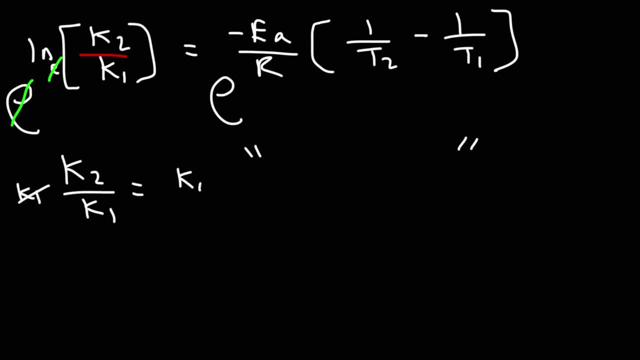 Now if we multiply both sides by K1. We can get an expression for K2.. So you want to write down this formula, because sometimes You need to calculate a new rate constant at a new temperature, So that new rate constant K2 is equal to K1 times E raised to the negative Ea over R, times 1 over T2, minus 1 over T1. 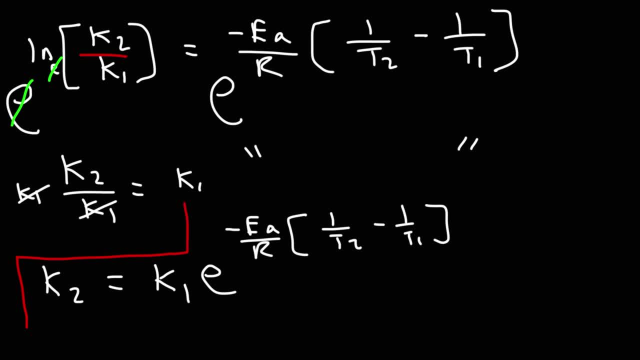 So this is the second equation that you want to write down. So you have an equation that will help you to calculate the activation energy, And this equation will help you to calculate the new rate constant given a new temperature. Now let's go back to the equation that we started with on this screen. 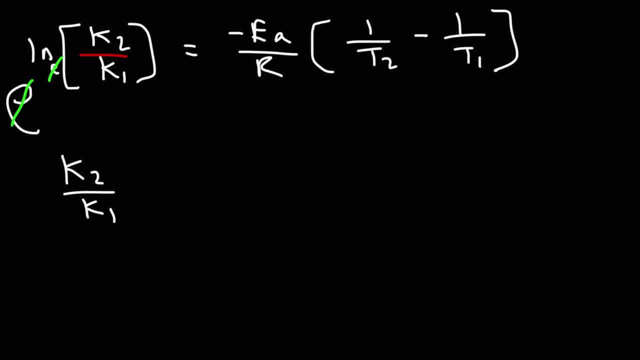 All right, that's as far as my software will. let me go back Now. sometimes you need to calculate the second temperature. So what we're going to do is We're going to isolate T2.. To do that, we're going to multiply both sides by negative R over Ea. 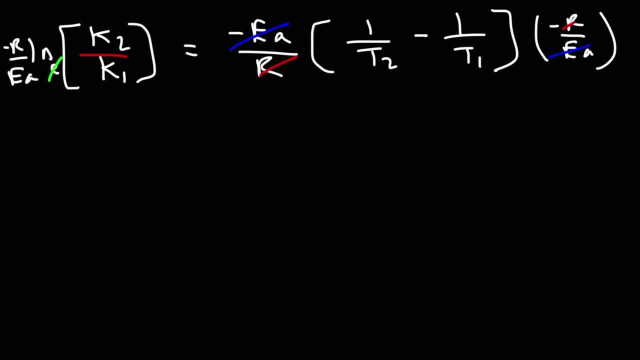 So those will cancel And we're going to have negative R Ln. K2 divided by K1 over Ea, That's going to equal 1 over T2.. Minus 1 over T1.. So we're going to move this to the other side, where it will become positive. 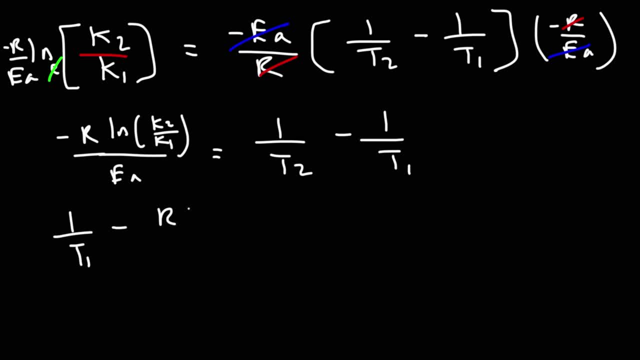 So we have 1 over T1, minus R, Ln, K2 over K1 over Ea. That's equal to 1 over T2.. Now we're going to raise both sides to the minus 1.. 1 over T2. raised to the negative 1 power is just T2.. 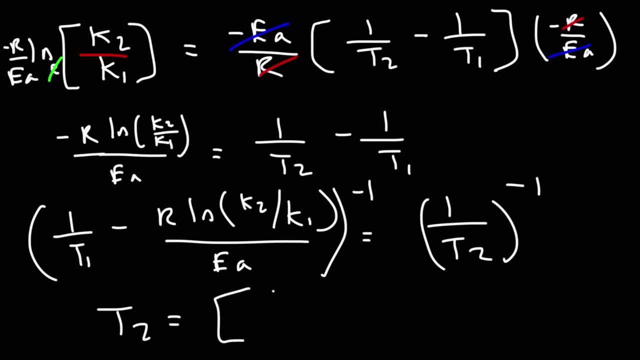 So we get this equation: T2 is equal to 1 over T1, minus R, Ln, K2 over K1 over Ea And this is raised to the negative 1 power. So this will help you to calculate the second temperature, If you know the second rate constant. 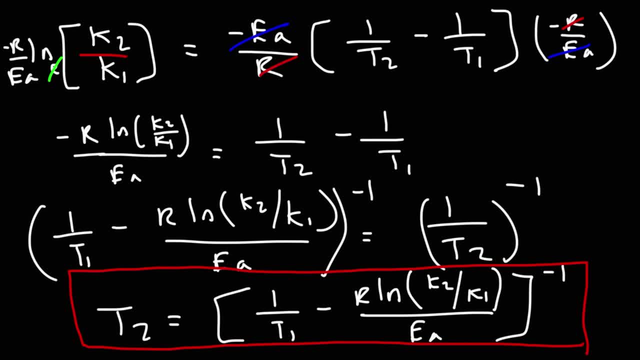 And, if you know, the activation energy. So those are some formulas that you want to use When solving problems associated with the Arrhenius equation: Activation energy, The rate constant And things like that. Now let's go ahead and put these equations to good use. 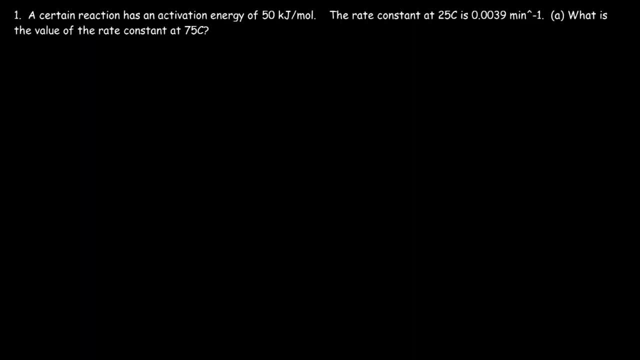 So we're going to work on a few practice problems. So take this one for example. A certain reaction has an activation energy of 50 kJ per mole. The rate constant at 25 degrees Celsius is 0.0039 minutes to the minus 1.. 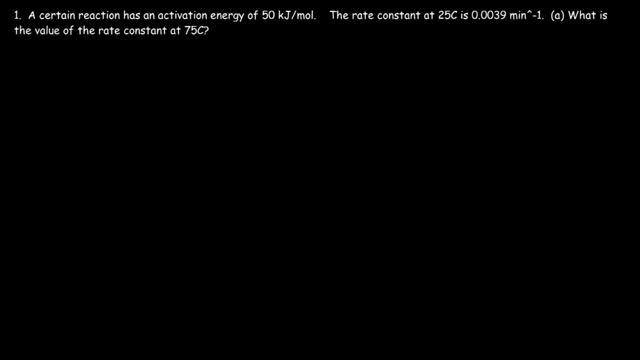 What is the value of the rate constant at 75 degrees Celsius? So first Let's make a list of what we know. So we have the activation energy: It's 50 kJ per mole. The rate constant, which we'll call K1, is 0.0039.. 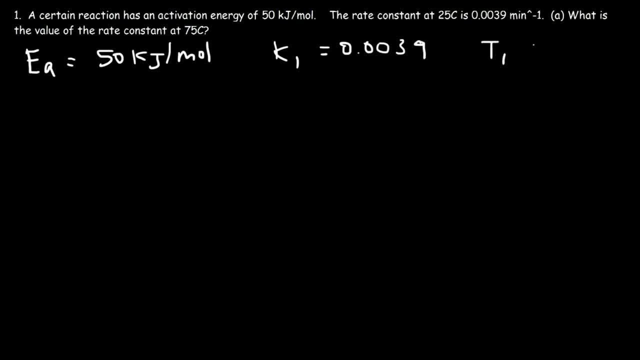 And that's at a temperature of 25 degrees Celsius, which we need to convert to Kelvin. So add 273 to 25.. That gives you 298 Kelvin. Our goal is to calculate K2.. And the second temperature is 75.. 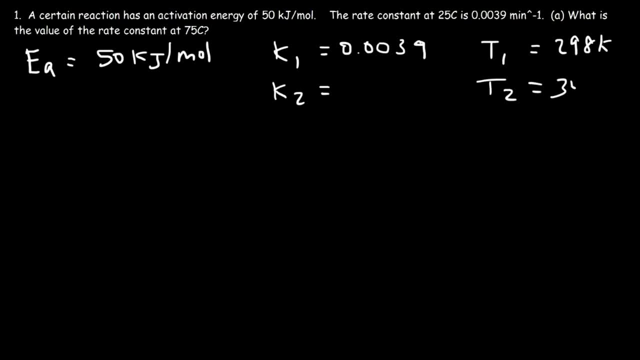 Plus 273.. So that's 348 Kelvin. So what is the formula that will help us to calculate K2?? It's K2 is equal to K1 times E raised to the negative EA over R, Multiplied by 1 over T2 minus 1 over T1.. 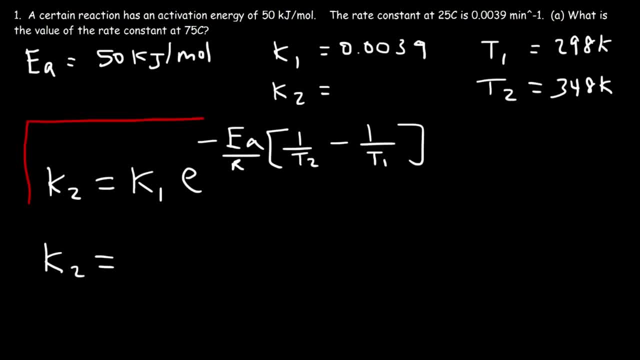 So anytime you need to find a rate constant at a different temperature, That's the formula that you want to commit to memory. Now, K1, we know it's 0.0039.. The activation energy has to be in Joules, So we've got to multiply 50 by 1,000.